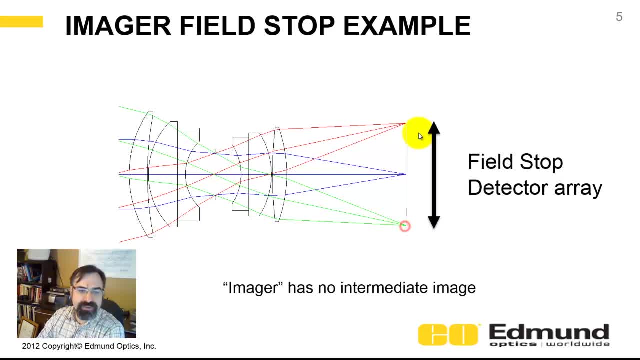 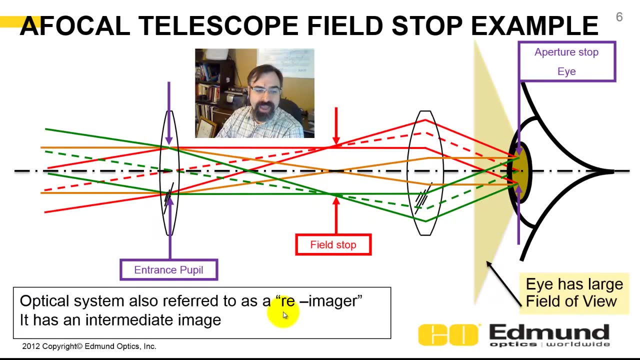 and this detector plane is going to be your field stop. And I make the distinction to say this is an imager because it does not have an intermediate image, And that distinction will become very important later. Now here is a case where we have a re-imager. 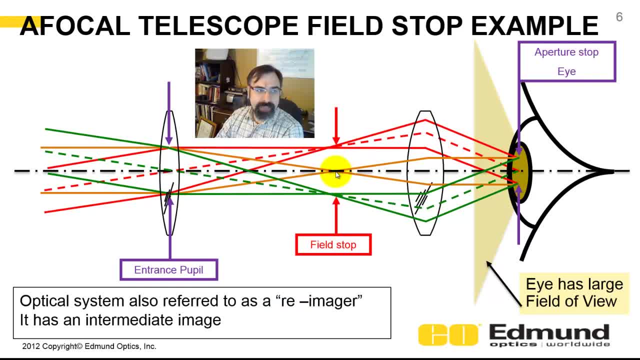 There is an intermediate stop here. This is a Keplerian, A focal, and you can see the detector in this case is your eye, this rather large eye, and the detector. your retina is huge. You have this huge field of view, this cone, right here. 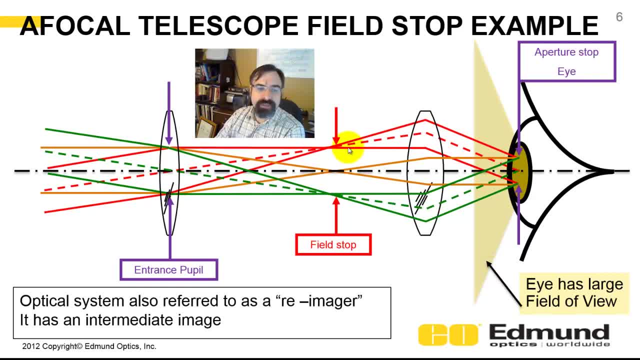 But that's not going to limit your field of view. Where this comes to an intermediate image, there'll be an aperture here and that would be your field stop. That limits how much you can see in the optical system And, again, because it's got an intermediate image, this could be called a re-imager. 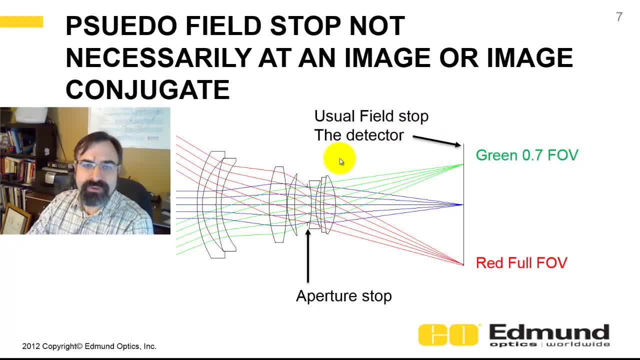 There could be other locations that limit your field, and I'm going to call these a pseudo-field stop, just for the lens design theorists that believe that your field stop is at an intermediate image. Here is a case where we have a wide field of view system. 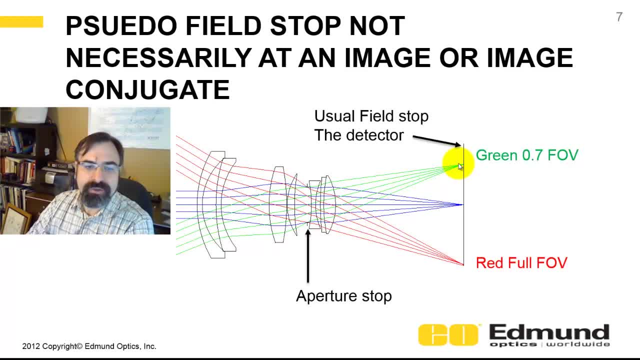 and this is at a Z-max. The blue rays are on axes, The green rays are positive- 0.707 field of view- And the red rays are negative- full field of view. And I'm changing the signs so we can see what's going on with the rays. 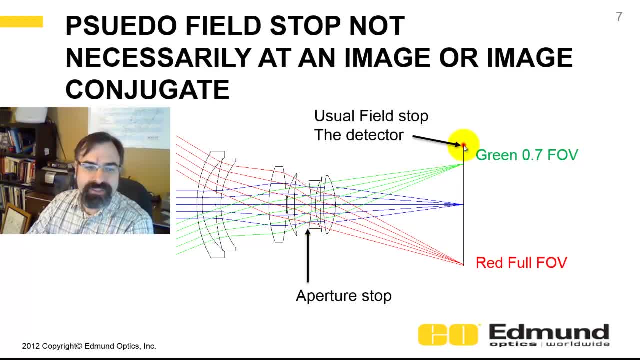 Your aperture stop is located here. Usually your field stop is the detector, but suppose you put an aperture up here For some reason. maybe you have to make this environmentally durable. it's going in space or it's going underwater and you've got a window right here that's going to block part of the green rays. 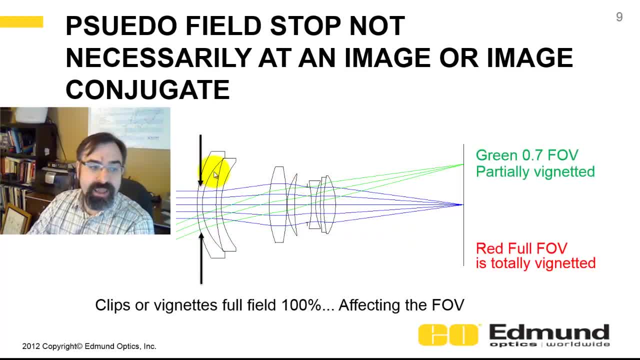 and in this case, all of the red rays. And you can see the red rays are totally vignetted, cutting your field down, whereas the green rays are partially vignetted. So this would be like another field stop or a pseudo-field stop. 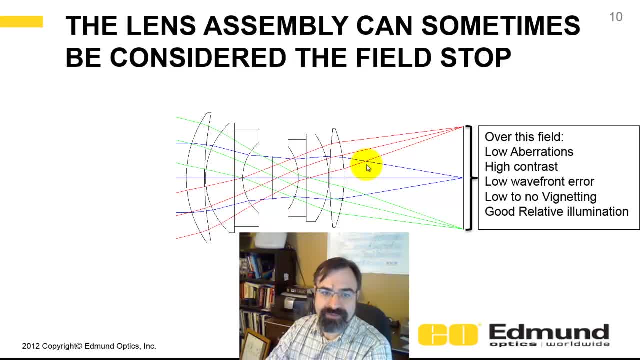 Sometimes you've got to consider the optical system as your field stop. For instance, let's suppose this double gauss is designed for one size detector or sensor, say half inch format or an 8mm image diameter. So this blue is the 8mm image diameter. 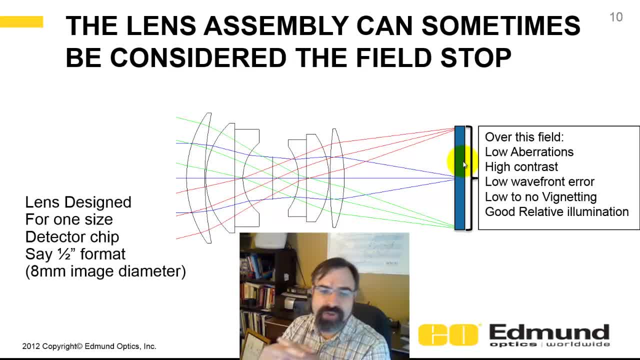 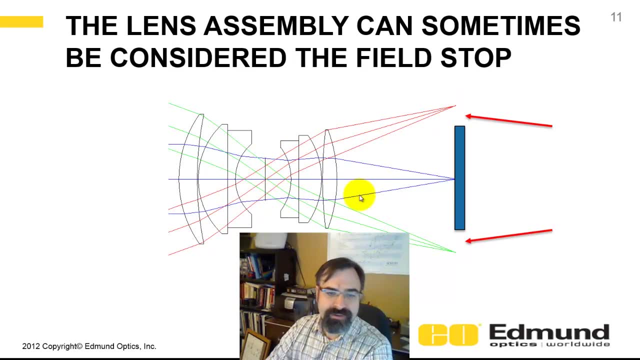 And over this field you've got low aberrations, high contrast, little wavefront error and no vignetting and good illumination. But suppose you buy this and match it with a larger detector, say outside here. Now, first you're going to see there's some vignetting here. 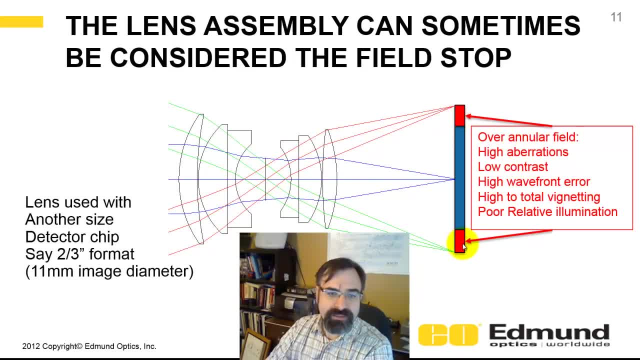 So over this annular ring- and let's suppose it's a larger format, say a 2 thirds inch format and that's an 11mm image diameter, This red annular ring, here you're going to have higher aberrations. 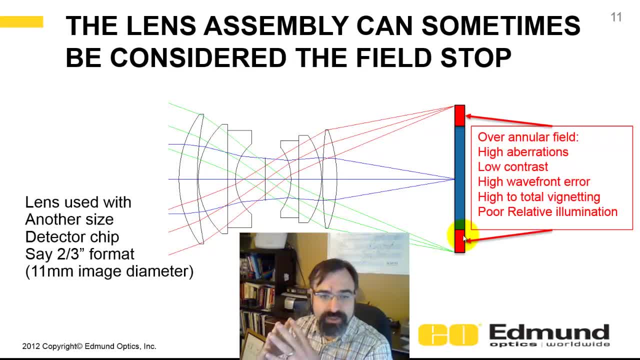 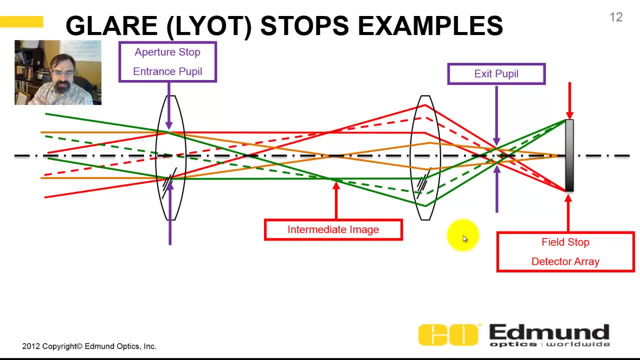 You may have higher aberrations, You have lower contrast And you could have poor illumination. So this is a case where you might consider your optics as limiting your field, not necessarily your field stop. There are cases now. this is a similar picture to the Keplerium. 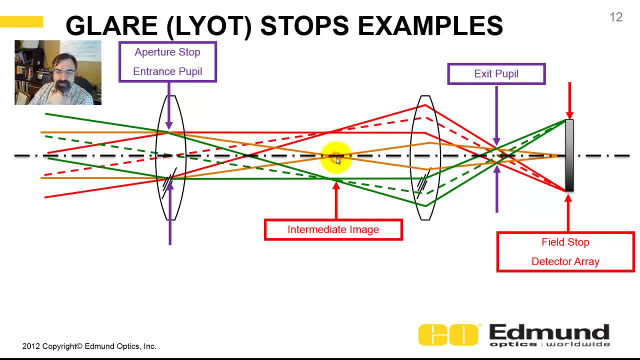 but this is coming to a focus and it's got an intermediate image. In this case, your detector array is your field stop, But you have an intermediate image here and I'm going to introduce the concept of a LEO stop or a glare stop. sometimes it's referred to as 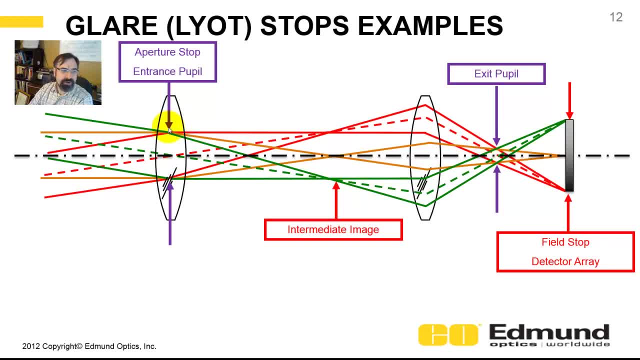 Your exit pupils up here and your entrance pupils on the front objective. Why would you put a stop here? Why would you put an aperture at the intermediate image? Well, there could be stray light sources outside your field of view- The sun. You're at a sports event. 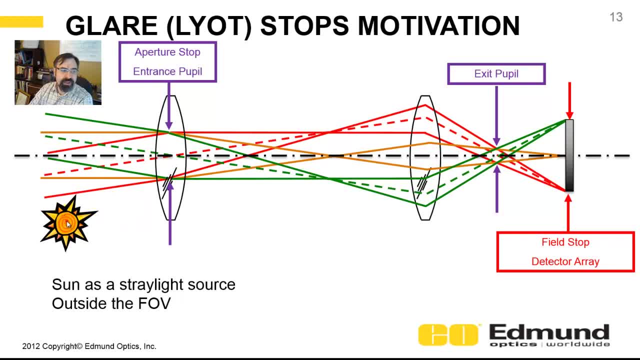 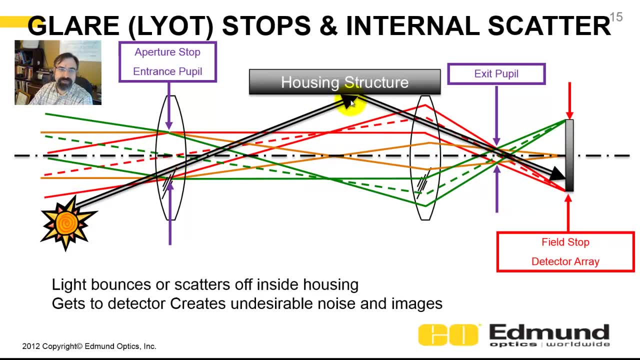 and there's large floodlights outside your field of view, This could cause stray light. So what happens is this light enters into the entrance pupil and gets into the optical system and it could bounce off some internal housing structure back to your detector and cause problems. 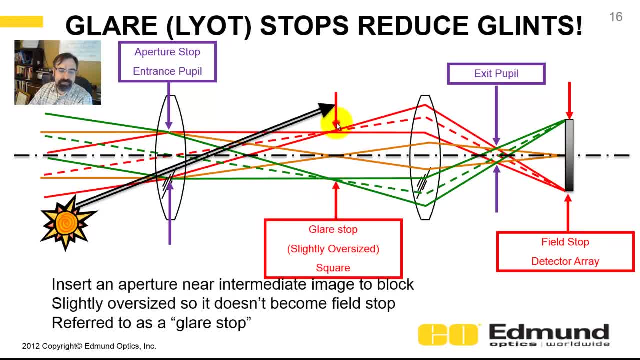 How do you avoid that? Well, if you put in an aperture stop. I'm sorry, if you put in an aperture here and you want to block that stray light that's called a glare or a LEO stop and you want to oversize that from the image. 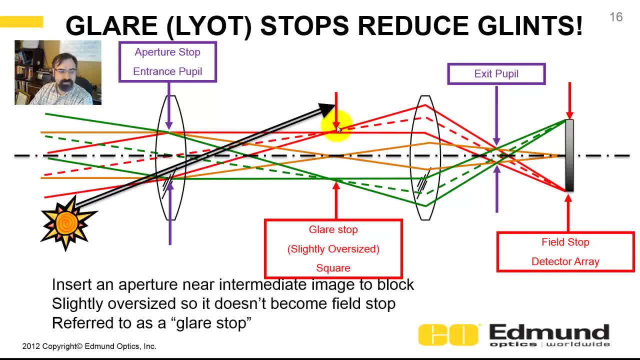 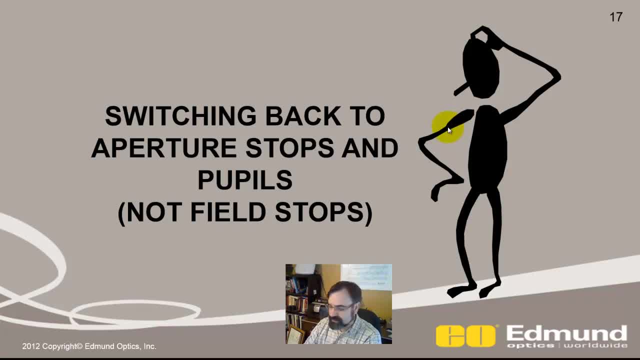 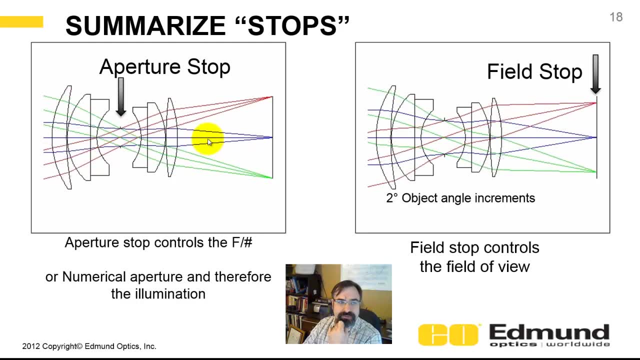 Because if you don't, then this becomes your field stop. Now I'm going to switch back to aperture stops and pupils. Previously, unless you're talking fields, I'm jumping back to apertures. There's some graphics showing the difference between an aperture stop and a field stop. 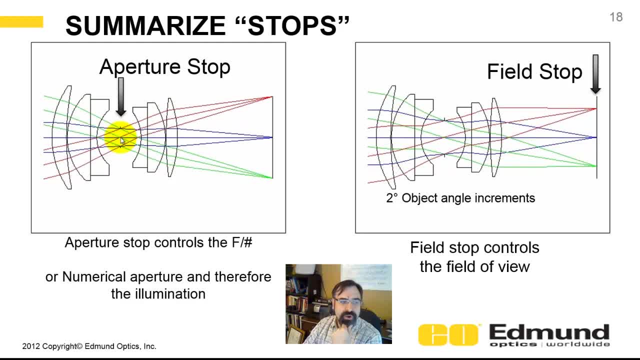 So on the left, we're changing the iris. The iris is growing and increasing and you can see that the F cone is varying, or the numerical aperture, and that's going to control your aberration balancing and it's going to control illumination. 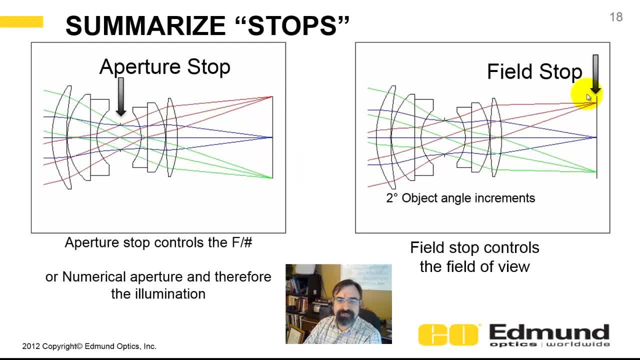 how much light gets back to your image plane As opposed to the field stop on the detector. it's going in and out and you can see that the field of view is increasing and decreasing If you look at the chief ray, say the green ray here. 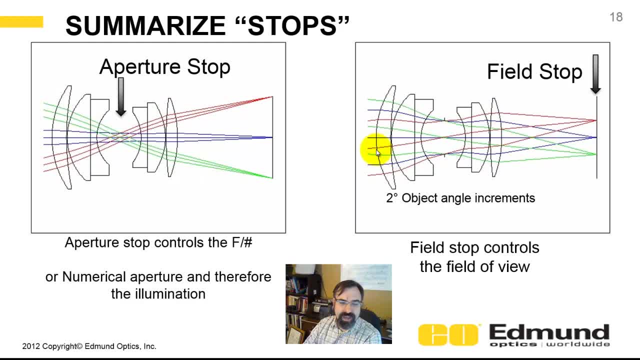 and I know it's moving around. it's going to be changing angle, So that's the distinction between an aperture and a field stop. I have these animated GIFs. My teenager makes fun. I always say it wrong. I've got these on my website if you want to hike them. 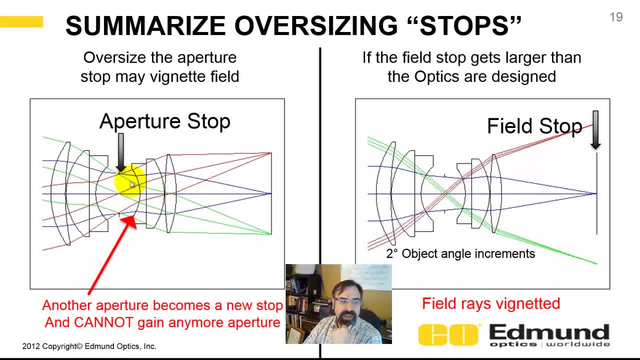 And likewise, if you oversize these stops on the left, if your aperture stop gets larger than it was designed for, you may hit a point where another aperture in the system becomes the aperture stop, And you can see in this double gauss. 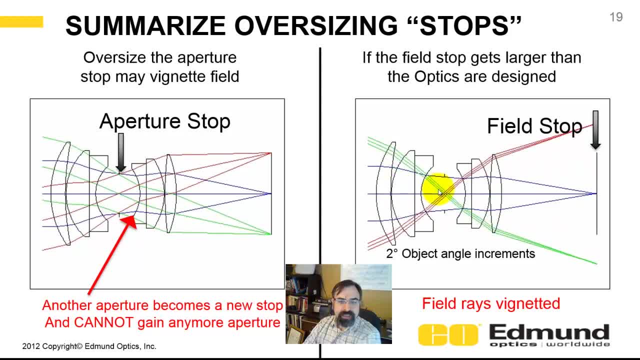 it might be the front of this flint right here And in a field: stop. if you increase the field you may end up with vignetting. You can see these F cones versus field are getting smaller. You're vignetting And there will be a limit. 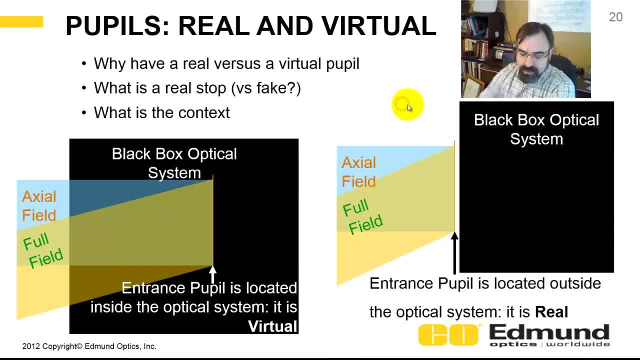 to how much field you can use. Pupils like images are going to have real and virtual pupils. So I was saying real images, real pupils at one point and someone said: well, what's a fake? Well, no, but the opposite of a real pupil. 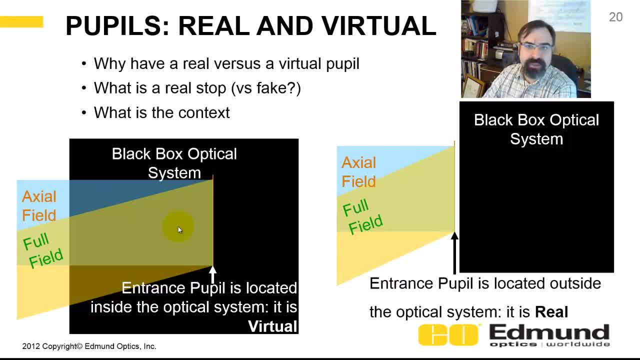 isn't a fake, it's a virtual. On the left, in the cases we've been looking at with the double gauss, you've got a virtual aperture. stop This, I'm sorry. a virtual entrance pupil. This entrance pupil is inside the optical system. 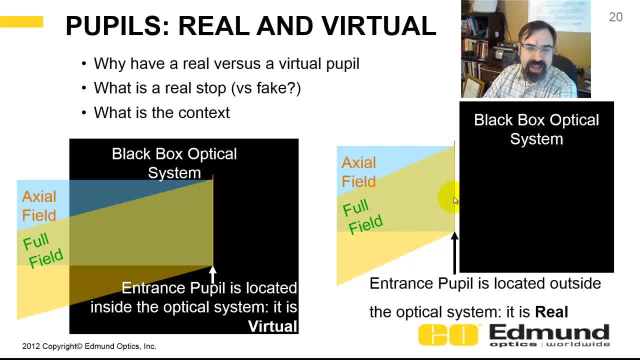 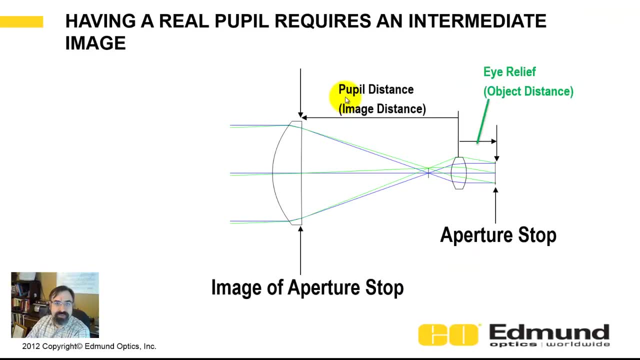 as opposed to a real pupil. It's located outside. In one case, you can't physically touch the virtual. You can't physically touch the pupil. In the real case you can. You can put an object there. So if you want a real pupil, 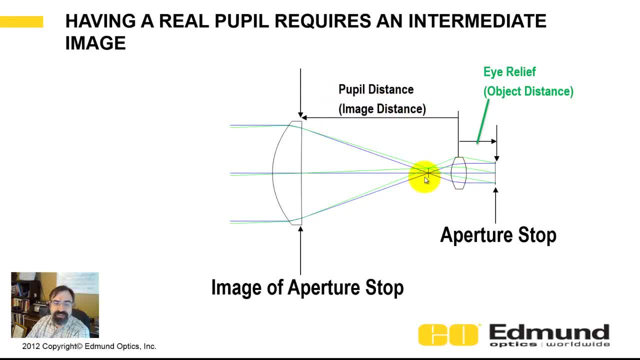 you're going to have to have an intermediate image. So here's a case of a Keplerian afocal, And let us suppose that the aperture stop is the eye And it's back here, So to find out where this pupil is located. 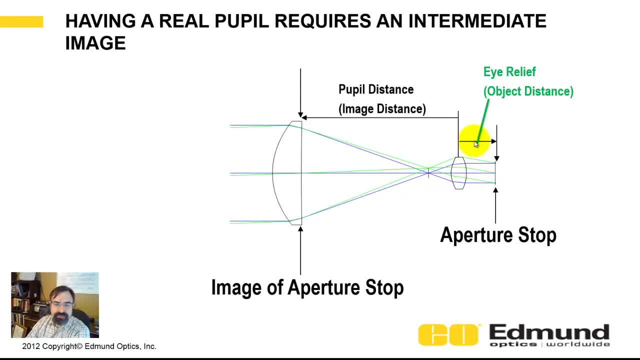 the distance from the stop to the eyepiece becomes the object, And then you use the imaging equations to locate where the pupil is. And I know we're going from right to left. We usually go left to right And if you take the objective away, 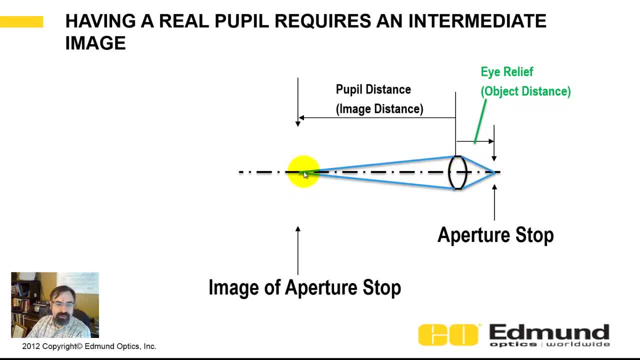 and you just look at this eyepiece. here are the rays drawn to show how to determine where the pupils are. You can use the lens maker's equation, where this is presented for a Cartesian coordinate system, Or you can use my favorite nomograph. 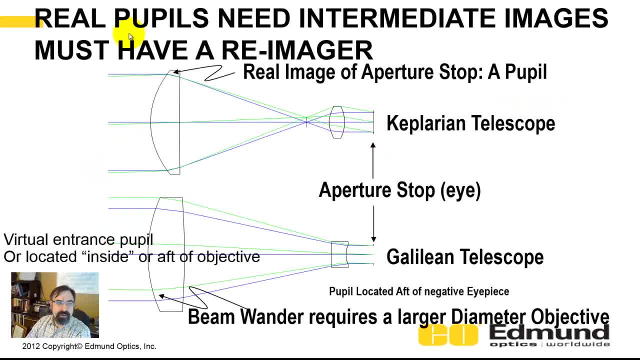 Imaging nomograph. Now real pupils. if you want a real pupil, I just want to hammer home: you need an intermediate image. So here is a case with this Keplerian: You have an aperture, stop in the back, You go through a positive eyepiece. 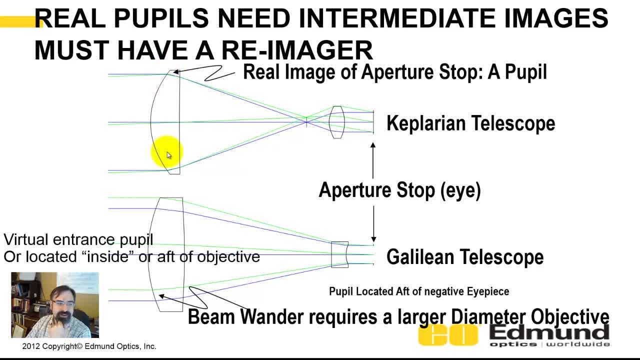 through an intermediate image into a real pupil And you can see that here, And having a pupil here is going to keep the diameter of this objective lens small, As opposed to a Gaussian a-focal. you have your eye pupil back here. the entrance pupil is virtual. 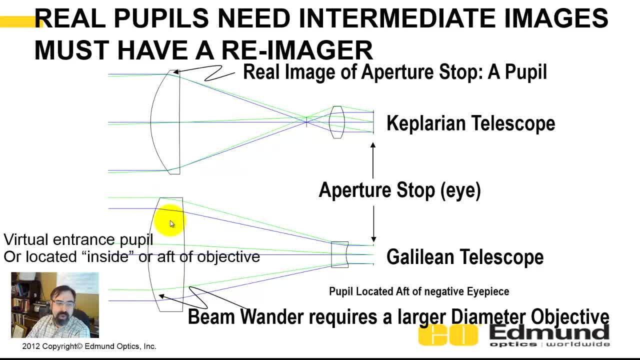 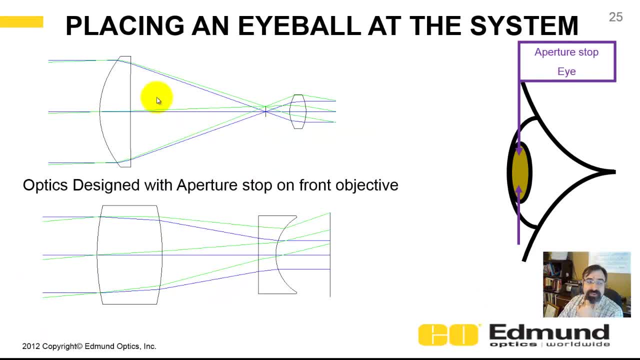 It's inside And you can see from the green to the blue rays. you're going to wander And that objective diameter is going to be much larger. Said another way, let us suppose that we've designed these systems so the eye, the iris, in your eye. 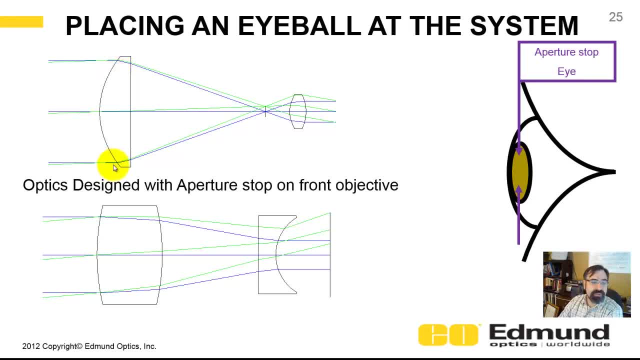 is not the limiting aperture, but the objective is. So in the Keplerian you're going to have an aperture- stop out here and it's going to come to a real pupil. And this is a case where, if you look at a like a rifle scope. 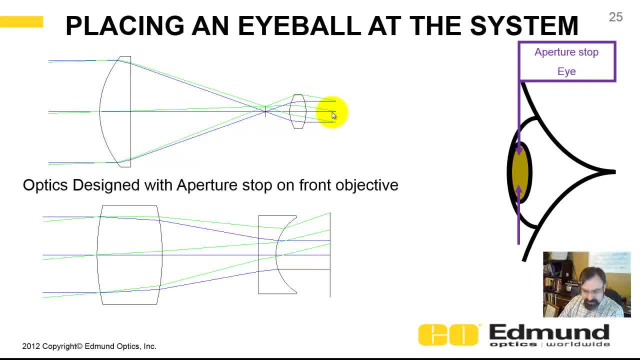 or a microscope objective. you can see there's a spot that you naturally put your eye on, As opposed to a Galilean. you can't do that. The pupil where your eye wants to go is virtual and you physically can't put your eye in that. 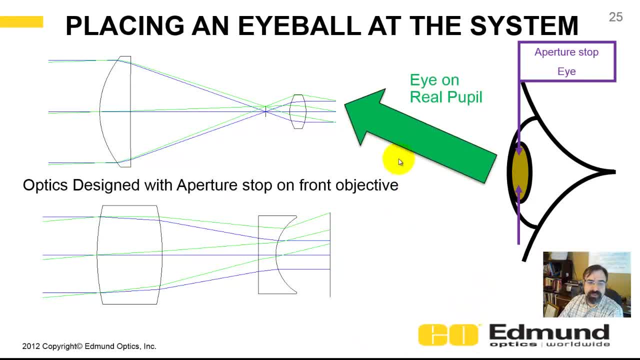 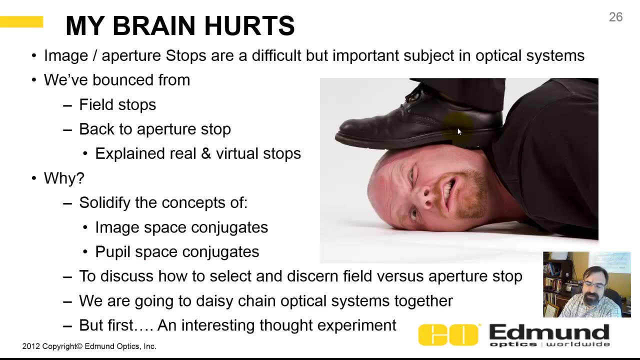 So that's the distinction between a real pupil and a virtual pupil, And I screwed up my animations here. I'm not going to go back and fix it, So this is just a picture to show my brain hurts. We bounced from stops field. 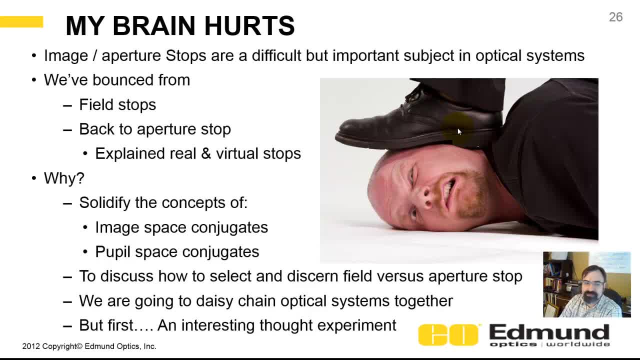 aperture, and we talked about real and virtual aperture stops. And why am I doing that? Well, I want to solidify the concepts of pupils in image and entrance space And I want to teach you when you look at an optical system. 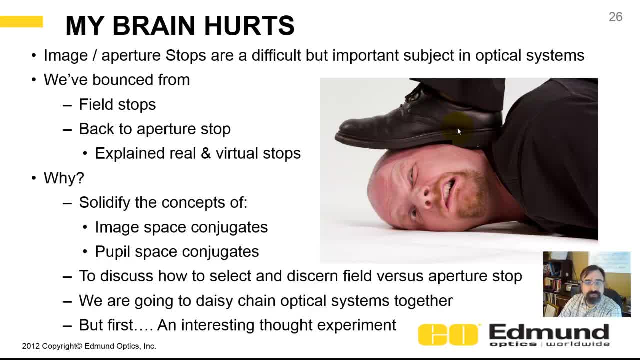 to tell what's the field stop, what's the aperture stop, so you can rapidly discern what the system is doing. And we're going to do that by daisy-chaining optical systems together. But first I want to run a thought experiment. 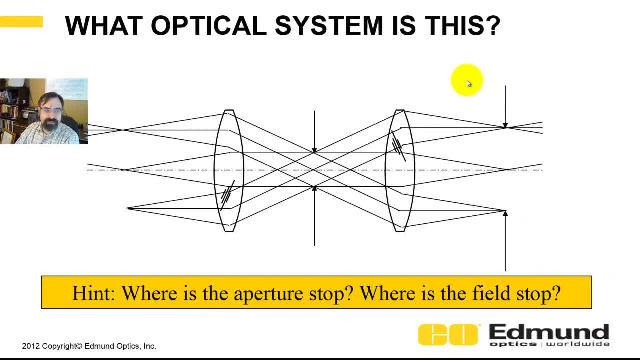 Here's a layout of a system And I'll ask you- and I'll leave this up for a little bit- what is this optical system? And, as a hint, you want to ask yourself: where's the aperture stop, Where is the field stop? 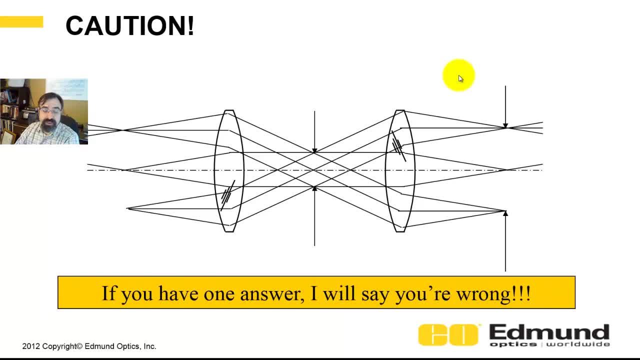 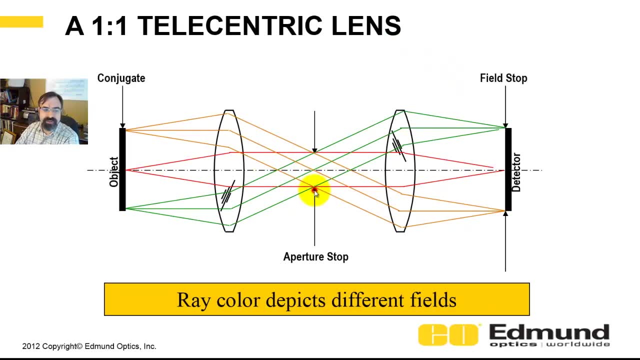 Now I'll give you some caution. This is a trick question. If you have only one answer, I'm going to say you're wrong. Because let's suppose you say it's a one-to-one telecentric. the center is the aperture stop. 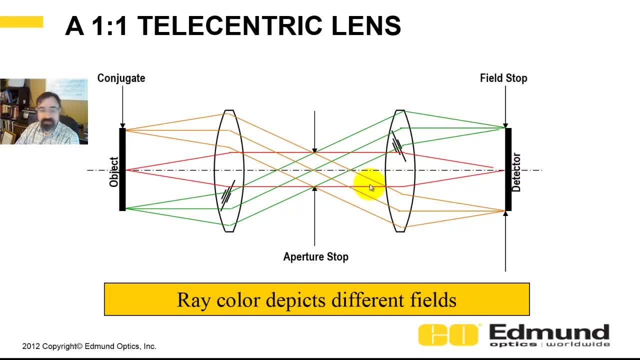 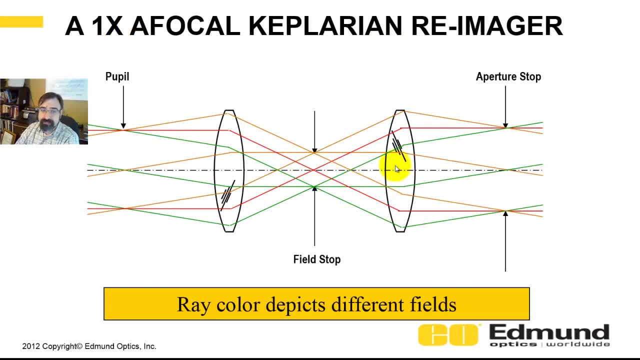 on the right is the detector, and ray color depicts different fields. If you say that's the answer, I'll say you're wrong, because it's really a one-to-one. a focal Keplerian where the center is a field stop. 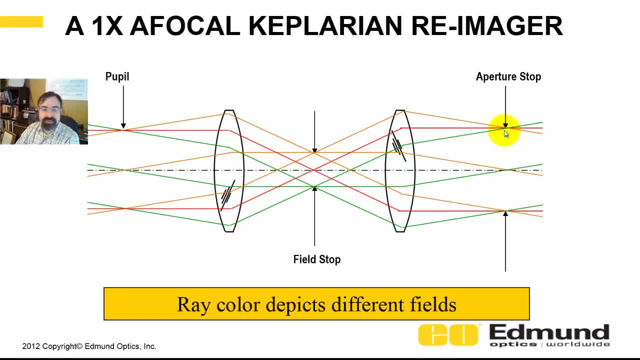 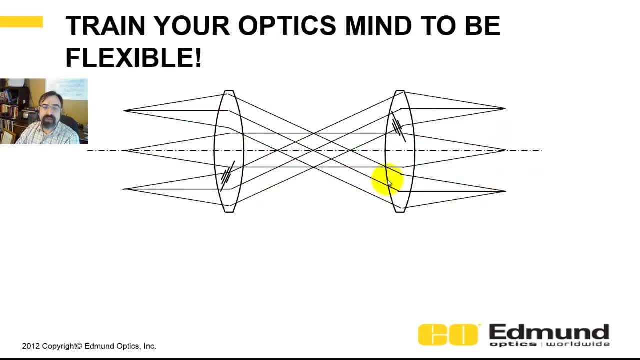 and the right is an aperture. stop. Again, color depicts different fields, So you need to train your mind to be flexible and understand what the original intent of the optical system is. So all of these pictures here are two different images And, of course, 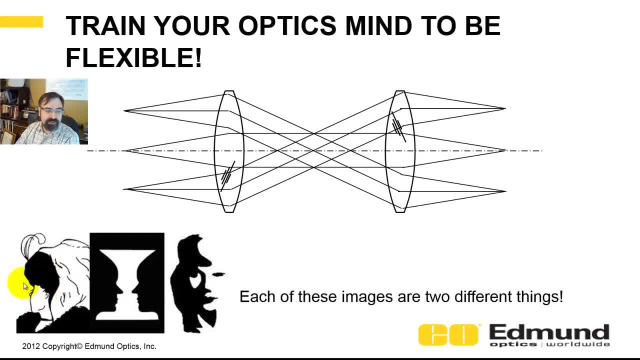 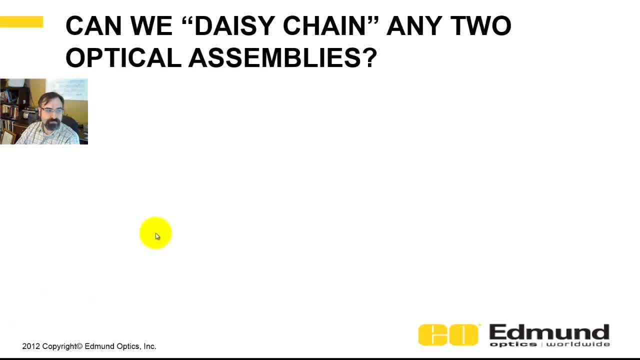 the famous one is this picture of a young lady looking out of the plane or an old lady looking looking into the, looking down to the left. So the question now is: can we daisy chain two optical systems together, Let's say a double Gauss? 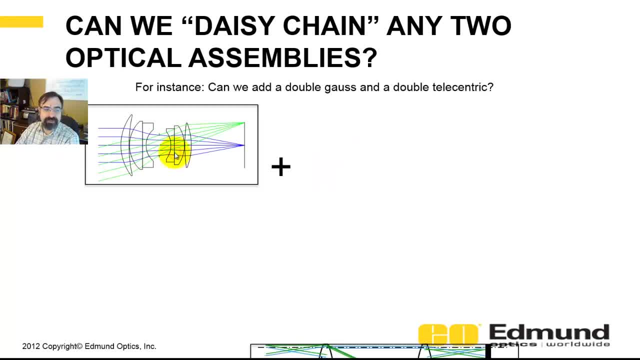 and a double telecentric system. So here's a double Gauss and here's a double telecentric. Does this work? What does it equal? And hopefully we could say the system focal length is just simply the double Gauss focal length. 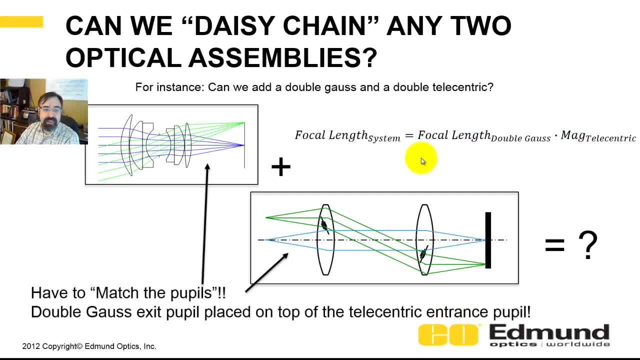 times the magnification of the telecentric. This only works if you match the pupils. In other words, you place the exit pupil of the double Gauss onto the entrance pupil of the telecentric. Said another way, you want to match these chief ray angles. 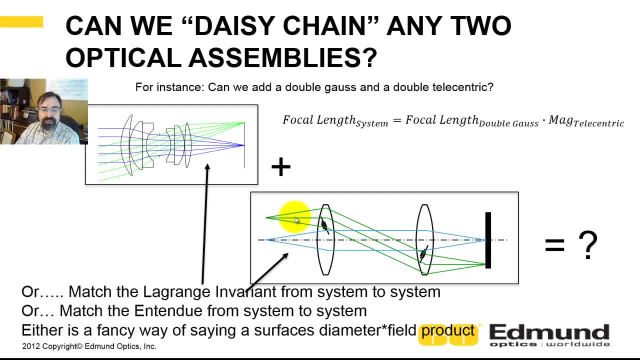 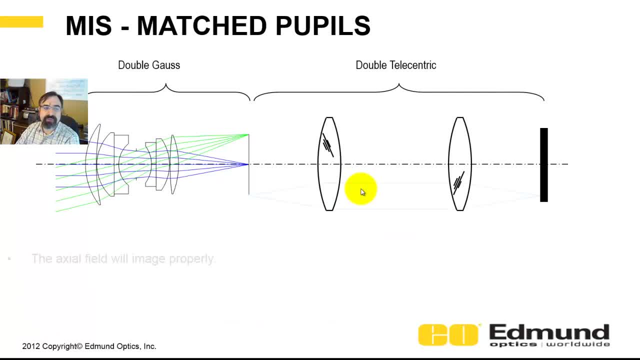 and I'm showing them here in red and notice they're not matched. Said another way, you've got to match the Lagrange and Altan. do So. let's give an example of a mismatched pupil On axis. everything's going to be fine. 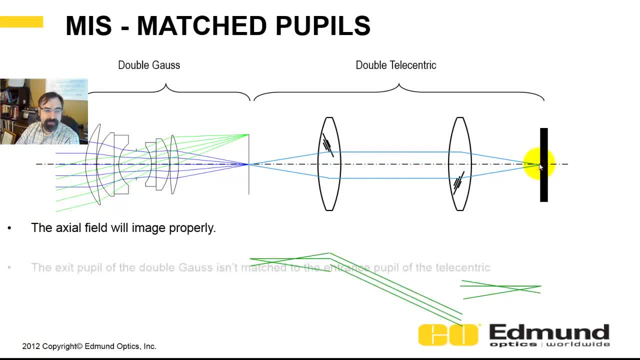 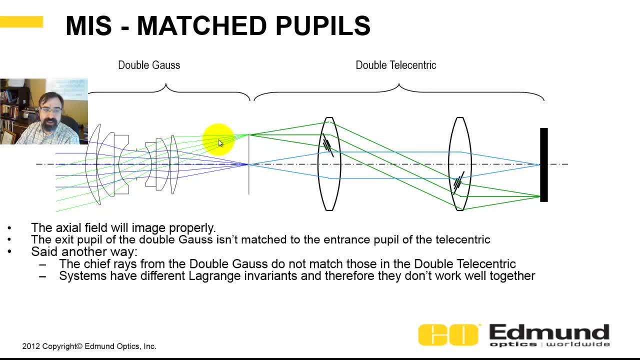 It's going to work. You get a nice on-axis image through. When you go off-axis again, you need to match these pupils and these chief rays And in this case, this thing I'm showing here- this is not happening. 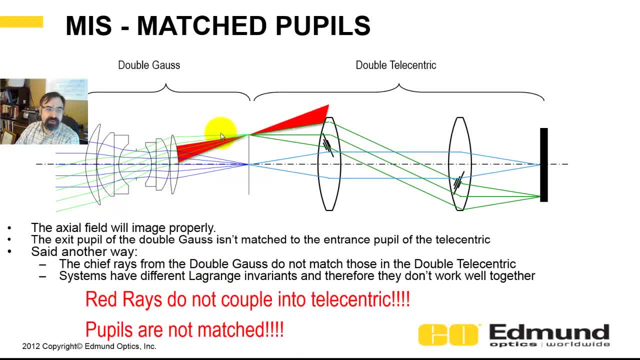 So what happens? We're not matching. I'm drawing these triangles. This red triangle here is showing that it's not going to couple into the double telecentric. So everything right here, all that light, is simply going to be lost. 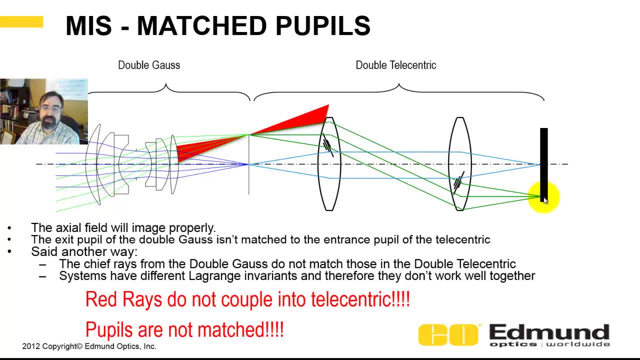 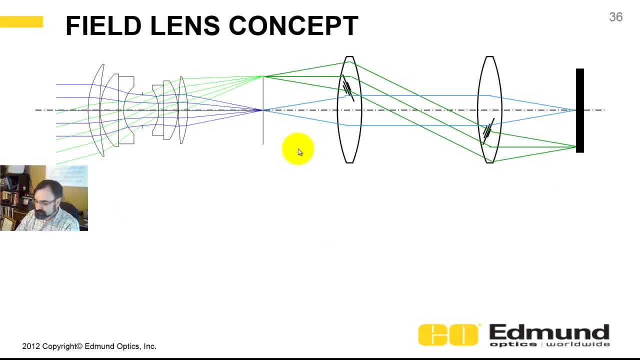 You're going to have low light illumination down on the edge of the detector. You can increase or decrease aberrations and change your optical performance as well. How do you get around this? Well, if you put a field lens right at the intermediate image. 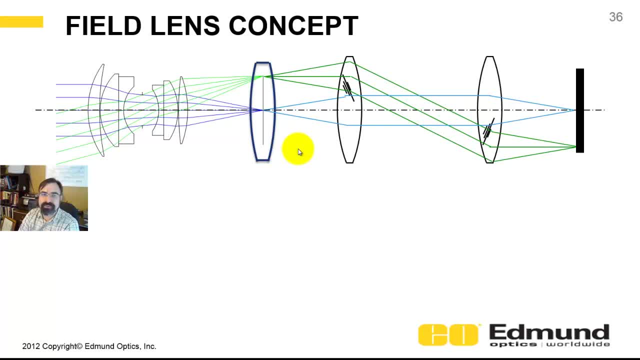 you can use this lens to relay or to image the pupils from one to the other, So the double gauss exit pupil is saved right here. Take the double gauss away and now you can see the lens is some distance d away from the exit pupil. 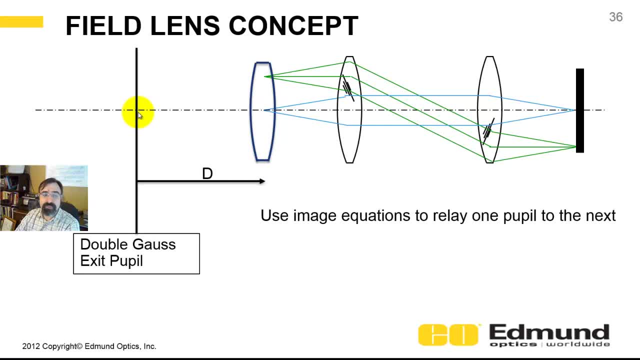 And now you just use the imaging equations to put this pupil onto where the telecentric is. Now this is a simple case, because the telecentric, by definition the pupil- is at infinity. So this field lens, in this case, just has to collimate the pupil. 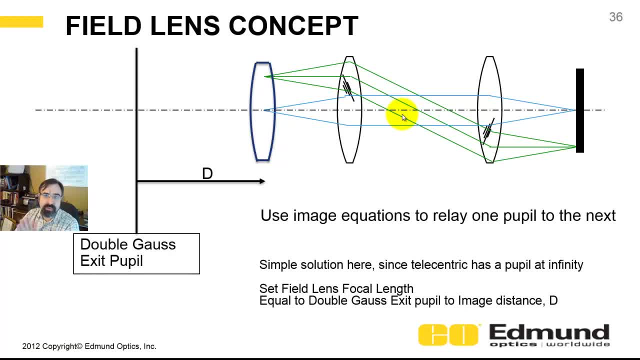 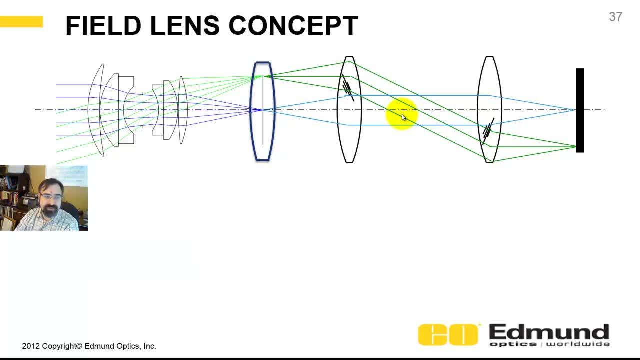 So the focal length of this particular field lens has to be whatever that distance. d is Very simple. So when you do that, you couple all your light in and at the edge of the field. Does this change the system focal length? No, it doesn't. 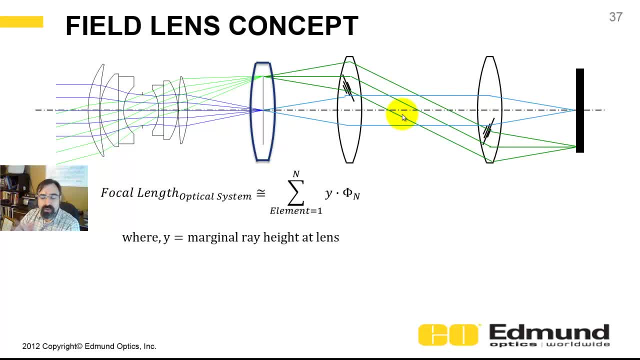 because the system focal length is proportional roughly to the power of each lens times the marginal ray height, And in this case the marginal ray height is zero. So this could be a short or a very long focal length, and it's not going to change. 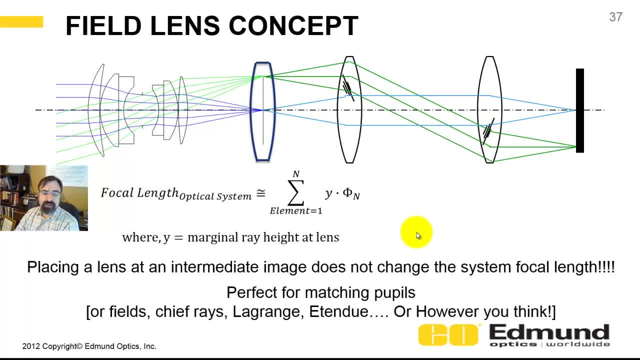 your optical system focal length. There's some caveats. If there's some scratches or dust on the field lens, they may be imaged right onto your detector. It could cause poor image quality If you're using this in a high-power laser. 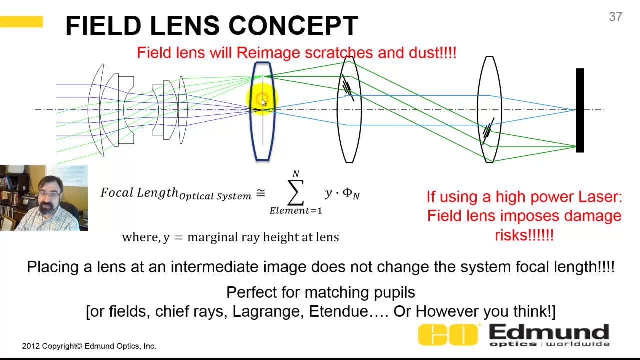 and you're focusing this high-power laser into an optical media, you could blow your lens And, in addition, putting this lens here is going to change the balance of field curvature through these systems, And we'll discuss what that is in upcoming videos. 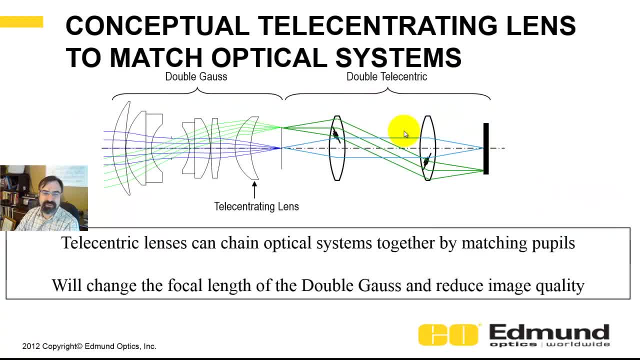 In some cases you want to change your field curvature effectively, A way around the problems with the field lens and putting it at an image. you could just put a telecentrating lens. In the last video we talked how to do that, so I'm not going to. 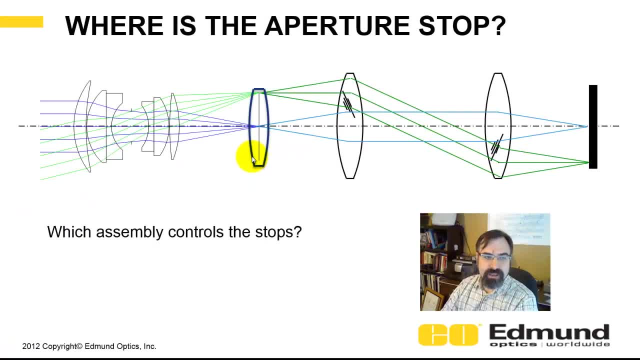 exasperate you both too much. So in this case, I want to ask you: where are the stops? And I really wish you'd take aperture out. So what system, which assembly controls the stops? You've got to worry about the field stop. 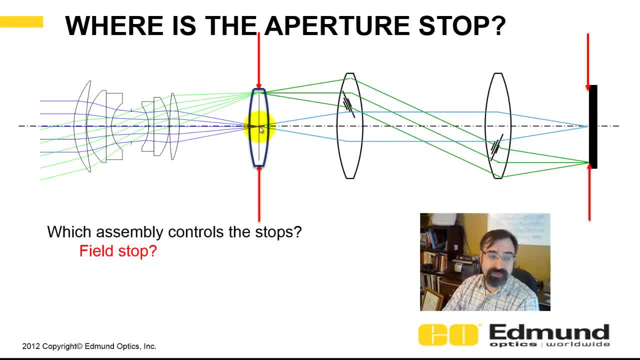 In this case, you could have the detector or you could have this field lens And the aperture stop. you could have an iris and the double telecentric, You can have an iris within the double gauss, And the answer is whichever clips or vignettes more. 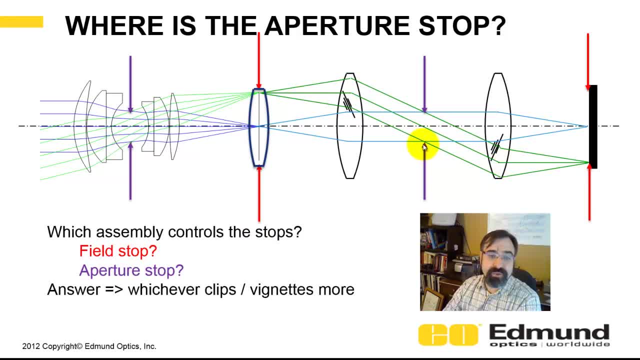 And this would be a cool system because you could use your detector as the field stop, And you might even want to put an iris back here to control stray light. Who knows, Or you undersize or oversize this lens to be, I'm sorry.